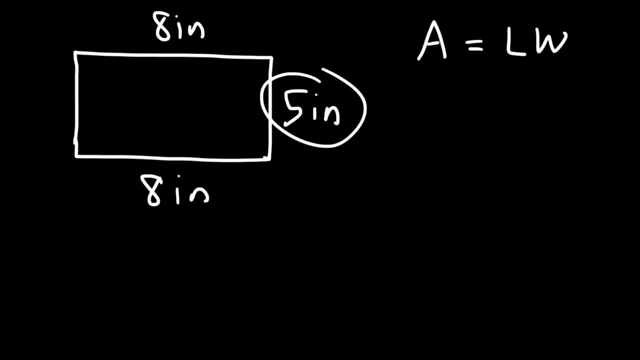 And if the right side is 5 inches, the left side must also be 5 inches, And so the formula for the perimeter of a rectangle it's 2L plus 2W, It's twice the value of the left, which is going to be 2 times 8 plus 2 times the width. 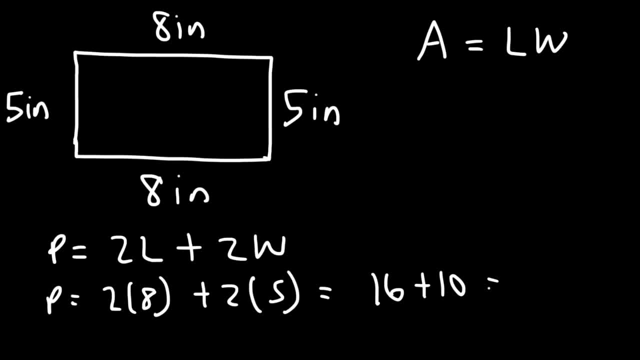 And so we're going to get 16 plus 10.. And so this is going to be 26 inches. It's not 26 square inches. So if you add up 8 inches plus 5 inches, that's going to be 13,, plus another 8 inches. that's 21 inches plus 5 again. 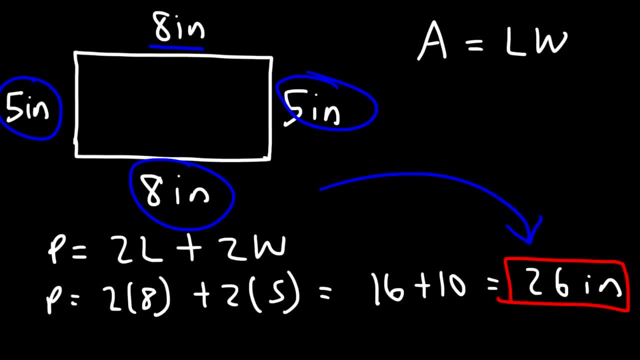 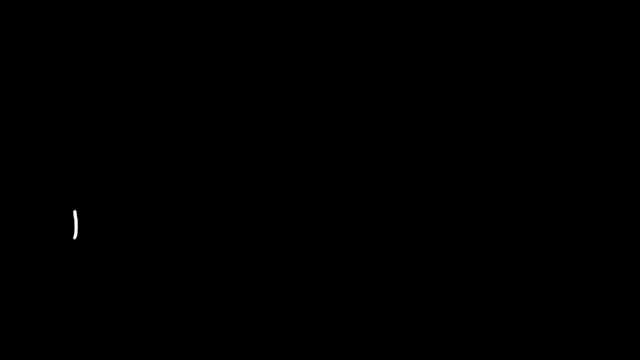 You're going to get a total of 26 inches, And so the perimeter is simply the distance around a figure, Whereas the area is basically the two-dimensional. So keep that in mind. Now for the next example, let's focus on the square. 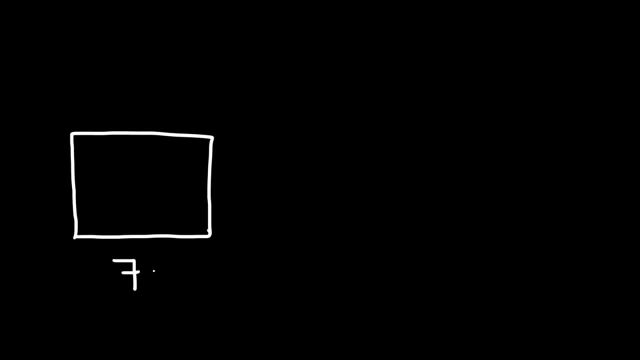 So let's say, if we have a square with a side length of 7 inches, What is the area and the perimeter of the square? Now, you need to know that all four sides of a square are the same, And so it's 7 inches all around. 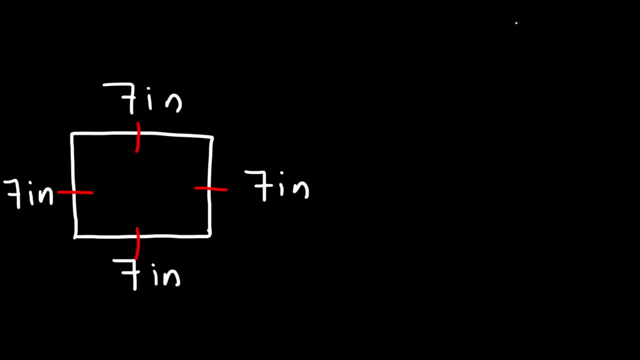 Now the area of the square is the perimeter of the square, And so it's 7 inches all around, And so the area of a square is similar to that of a rectangle. For a rectangle, it's left times width. For a square, all sides are the same. 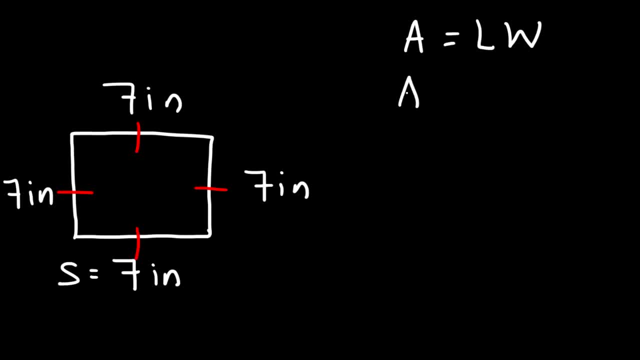 So let's call the side length S, So it would be S times S or simply S squared. So in this case, the area of this square is going to be 7 times 7, or 7 squared, which is 49 square inches. 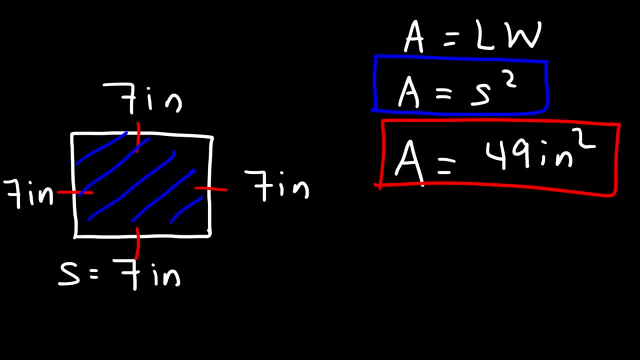 And so that's the first part For this problem. Now for the second part. we need to calculate the perimeter, And intuitively, we can see that it's going to be the sum of all four sides. Don't forget that the perimeter is the distance around the figure. 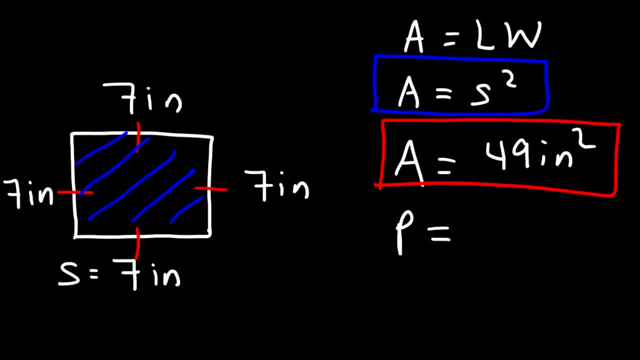 So it's going to be 7 plus 7 plus 7 plus 7, which is 28 inches. Or you could say S plus S plus S plus S, which is 4S, So it's 4 times 7.. 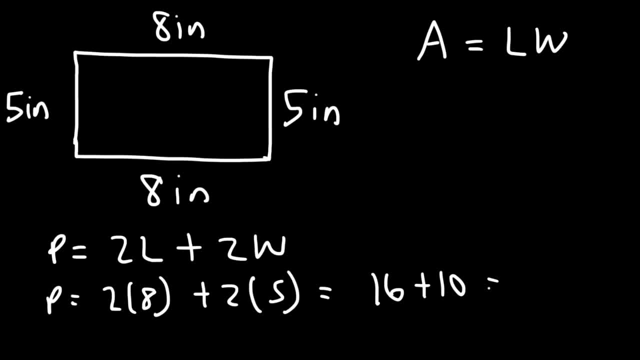 And so we're going to get 16 plus 10.. And so this is going to be 26 inches. It's not 26 square inches. So if you add up 8 inches plus 5 inches, that's going to be 13,, plus another 8 inches. that's 21 inches plus 5 again. 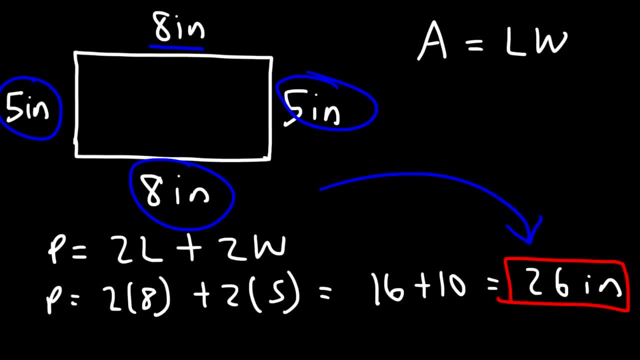 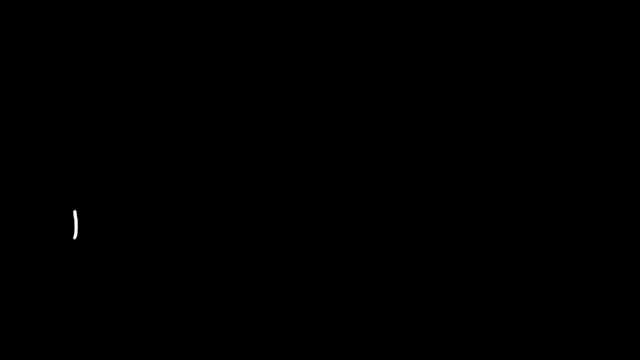 You're going to get a total of 26 inches, And so the perimeter is simply the distance around a figure, Whereas the area is basically the two-dimensional. So keep that in mind. Now for the next example, let's focus on the square. 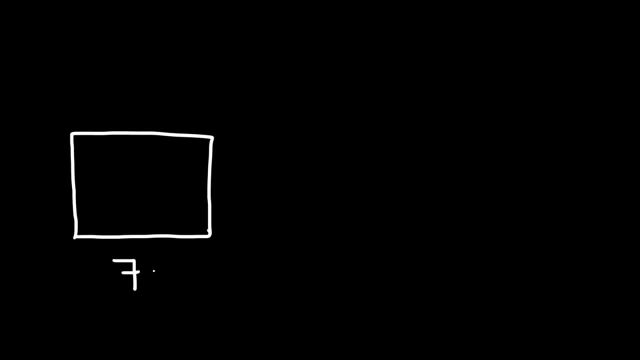 So let's say, if we have a square with a side left of 7 inches, What is the area and the perimeter of the square? Now, you need to know that all four sides of a square are the same, And so it's 7 inches all around. 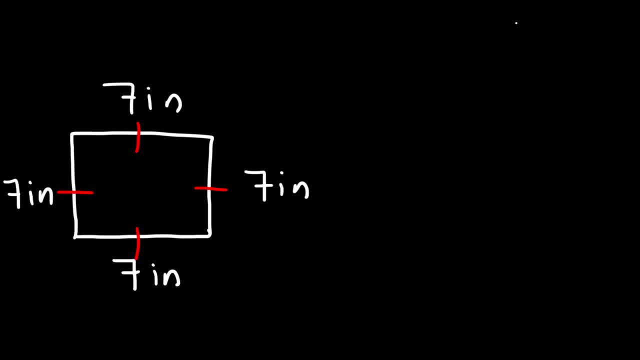 Now the area of the square is 7 inches, And so the area of a square is similar to that of a rectangle. For a rectangle, it's left times width. For a square, all sides are the same, So let's call the side left S. 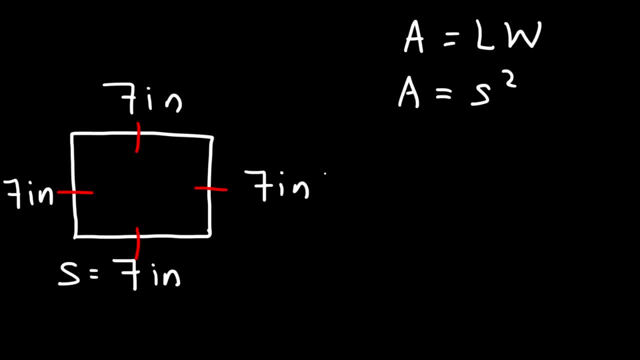 So it would be S times S or simply S squared. So in this case, the area of this square is going to be 7 times 7, or 7 squared, which is 49 square inches, And so that's the first part. 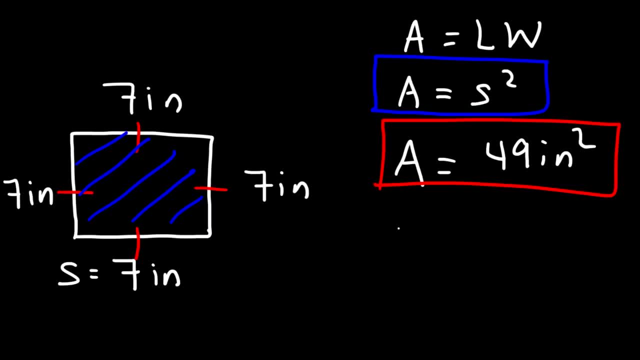 For this problem. Now for the second part. we need to calculate the perimeter And intuitively we could see that it's going to be the sum of all four sides. Don't forget that the perimeter is the distance around the figure, So it's going to be 7 plus 7 plus 7 plus 7, which is 28 inches. 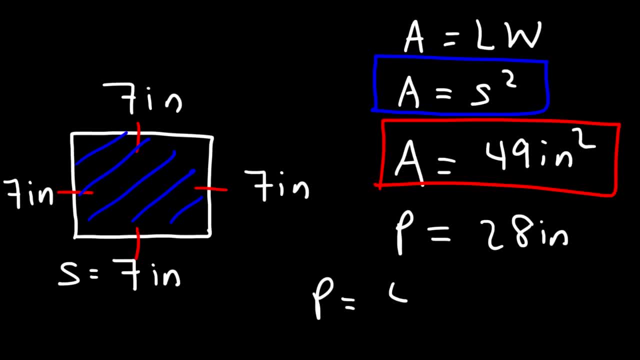 Or you could say S plus S, plus S plus S, which is 4S, So it's 4 times 7. Which will give us 28.. And so that's how you can find the perimeter of a square. Now let's work on some word problems. 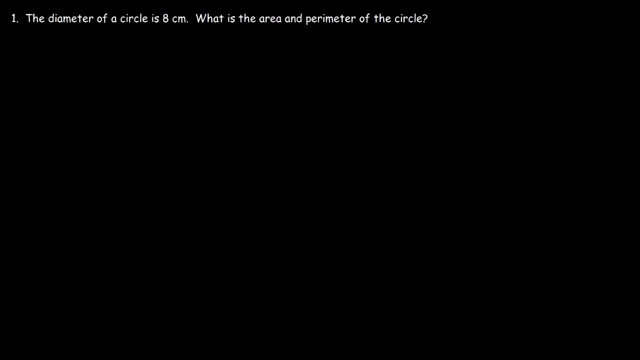 The diameter of a circle is 8 centimeters. What is the area and perimeter of the circle? So let's draw a picture. And so this is the diameter: It's 8 centimeters. How can we determine the area and the perimeter? 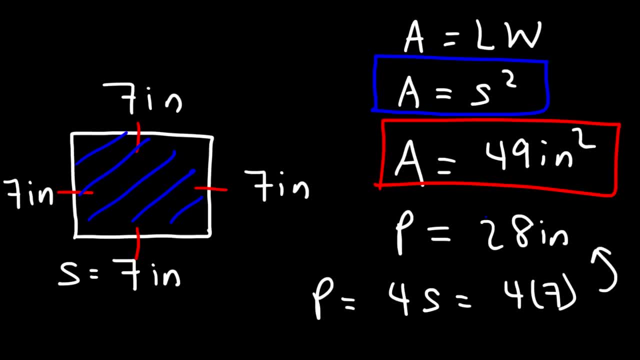 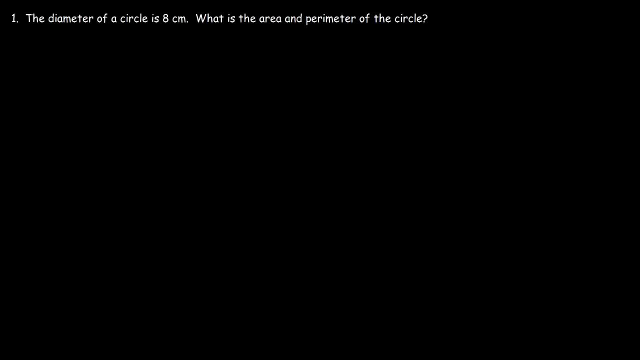 Which will give us 28.. And so that's how you can find the perimeter of a square. Now let's work on some word problems. The diameter of a circle is 8 centimeters. What is the area and perimeter of the circle? 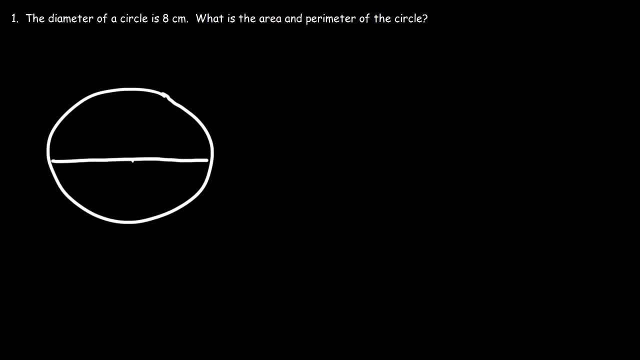 So let's draw a picture, And so this is the diameter. It's 8 centimeters. How can we determine the area and the perimeter? The first thing I would recommend doing is finding the radius. The radius is one half of the diameter. 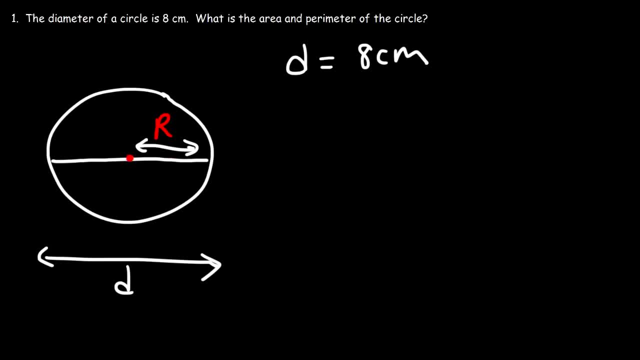 So this is the radius. It's the distance between the center of the circle and any point on the circle. So half of 8 is 4.. Therefore, the radius is 4.. Now to calculate the area of the circle, We could use this formula: 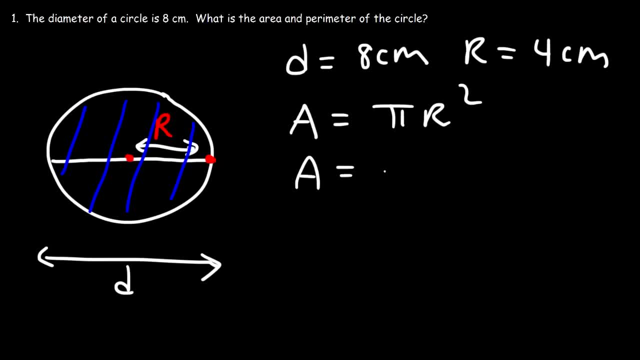 Area is pi r squared, So we're going to use this formula. So it's going to be pi times 4 squared, which is going to be 16 pi square centimeters, And so this is the area of the circle. Now, if you want to get the decimal value of that, I'm going to use the exact value for pi 3.141592654 times 16.. 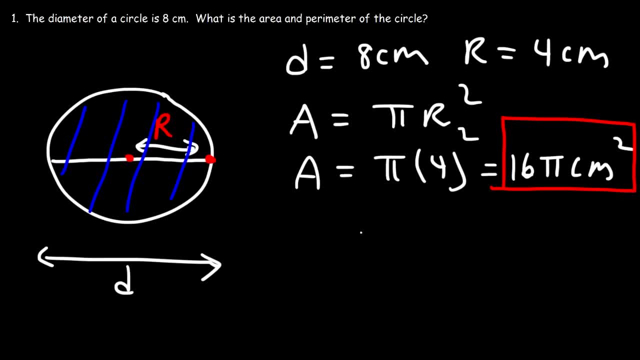 And so you should get 50.265 square centimeters for the area of the circle. Now, what about the perimeter of the circle? So how can we determine the distance around the circle? And there's a formula for that: It's basically the circumference, which is 2 pi r. 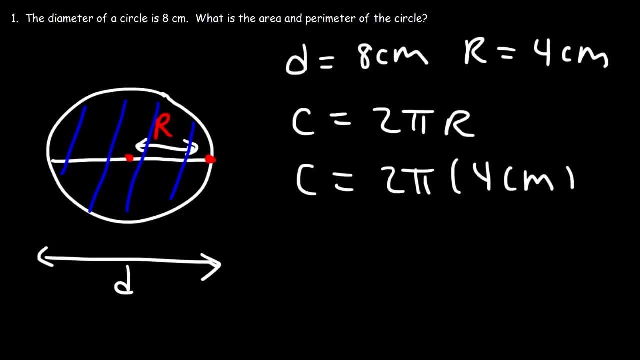 So it's going to be 2 pi times 4 centimeters, And so that comes out to be 8 pi centimeters, Which, if we convert that to a decimal number, that's going to be 25.133 centimeters. 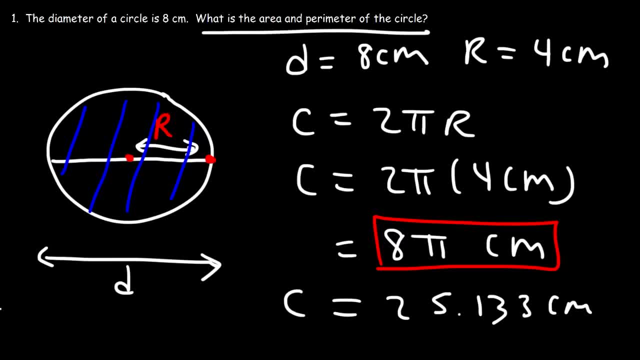 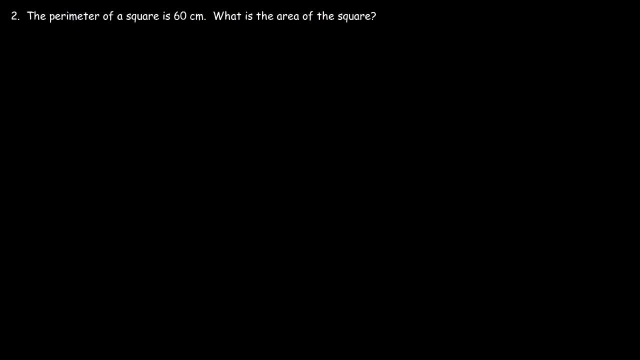 And so that's how you can find the area and the perimeter of the circle. The perimeter of the circle is simply called the circumference of the circle. Now here is another problem. The perimeter of a square is 60 centimeters. What is the area of the square? 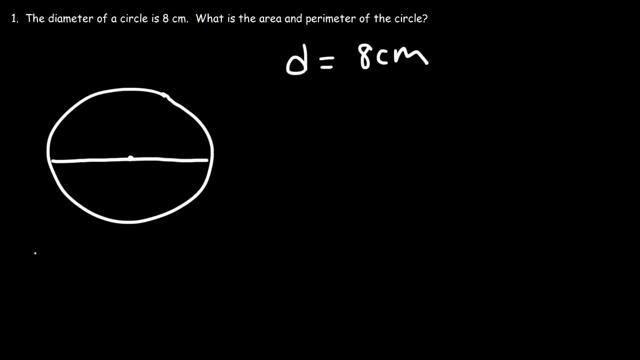 The first thing I would recommend doing is finding the radius. The radius is one half of the diameter, So this is the radius. It's the distance between the center of the circle and any point on the circle. So half of 8 is 4.. 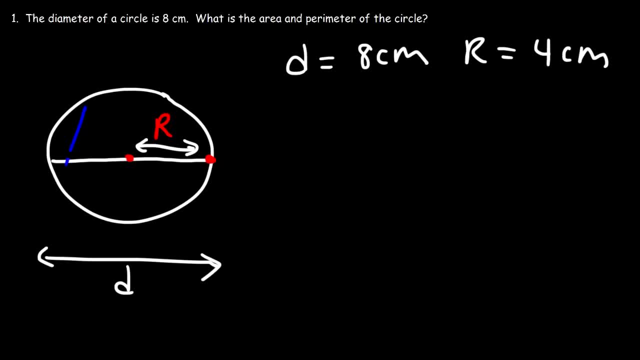 Therefore the radius is 4.. Now to calculate the area of the circle, we could use this formula: Area is pi r squared, So it's going to be pi times 4 squared, which is going to be 16 pi square centimeters. 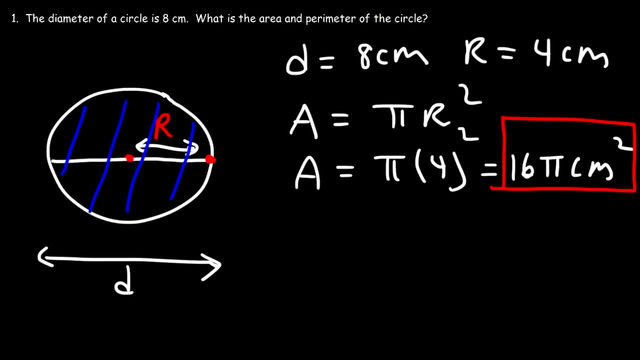 And so this is the area of the circle. Now, if you want to get the decimal value of that, I'm going to use the exact value for pi 3.141592654 times 16.. And so you should get 50.265 square centimeters for the area of the circle. 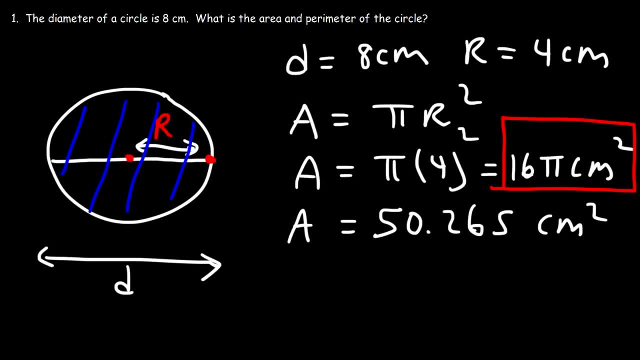 Now, what about the perimeter of the circle? So how can we determine the distance around the circle? And there's a formula for that: It's basically the circumference, which is 2 pi r, So it's going to be 2 pi times 4 centimeters. 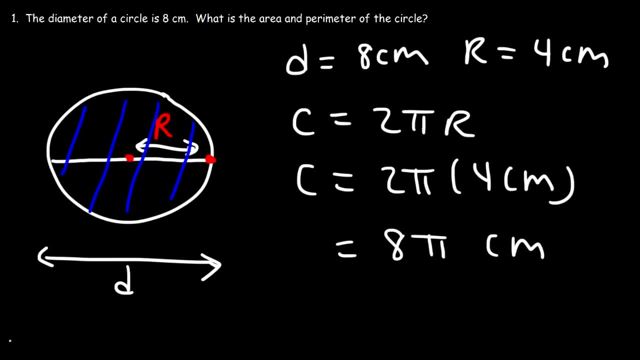 And so So that comes out to be 8 pi centimeters, Which if we convert that to a decimal number, that's going to be 25.133 centimeters. And so that's how you can find the area and the perimeter of the circle. 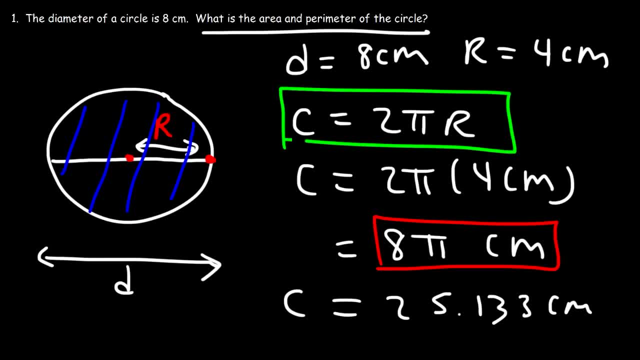 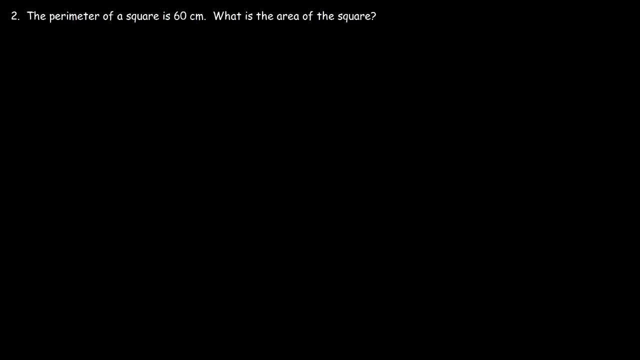 The perimeter of the circle is simply called the circumference of the circle. Now here is another problem. The perimeter of a square is 6. 60 centimeters. What is the area of the square? So how can we find the area if we're given the perimeter? 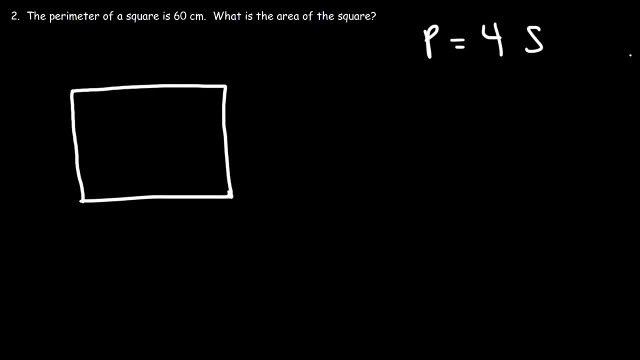 So first square, remember that the perimeter is 4 times the side length. So if the perimeter is 60, we could easily solve for the side length. We just got to divide both sides by 4.. And so 60 divided by 4 is 15.. 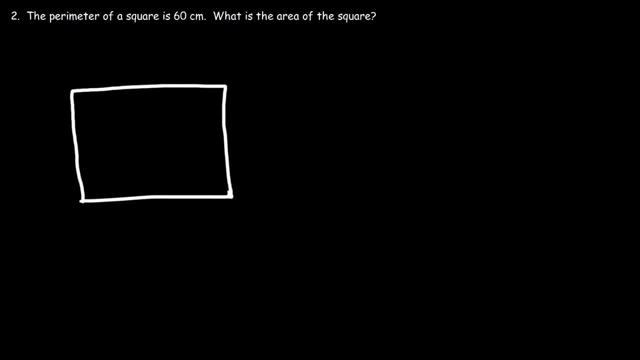 So how can we find the area if we're given the perimeter? So first remember that the perimeter is 4 times the side length. So if the perimeter is 60, we could easily solve for the side length. We just got to divide both sides by 4.. 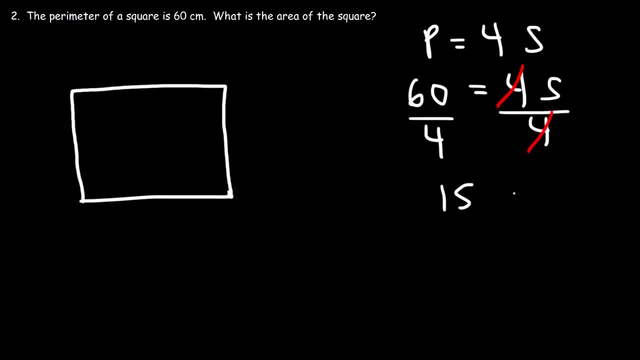 And so 60 divided by 4 is 15.. So therefore, the side length of the square is 15 centimeters all around. So now that we have the side length, we can calculate the area. So the area of this square is going to be S squared. 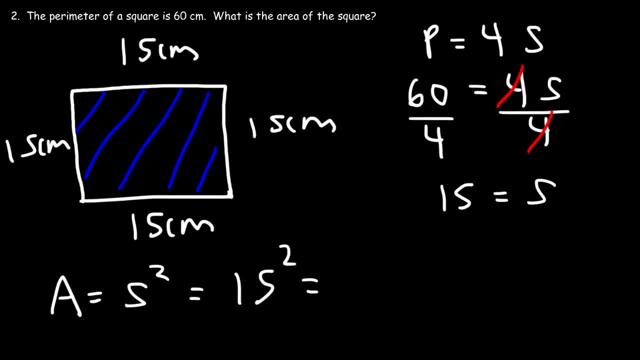 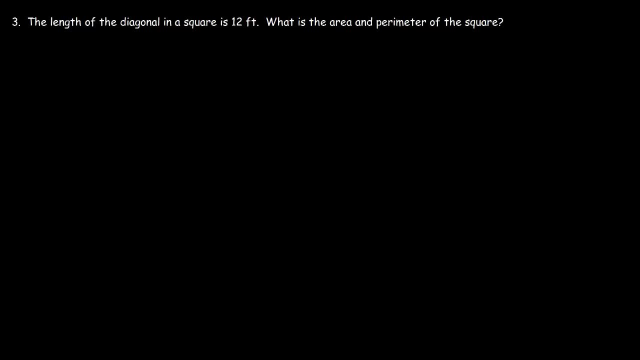 Or basically 15 times 15, which is 15 squared, And so that comes out to be 225.. square centimeters, And so that's it for this problem. That's the area of this particular square. Now let's try this problem. The length of the diagonal in a square is 12 feet. 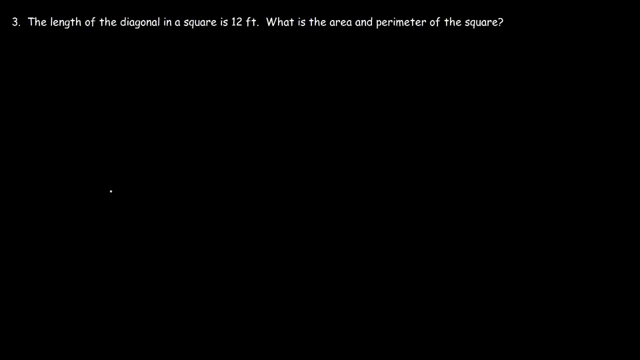 What is the area and perimeter of the square? So if we're given the length of the diagonal- let's call it L- How can we find the side length S? Notice that this forms a right triangle, And so we could use the Pythagorean theorem. 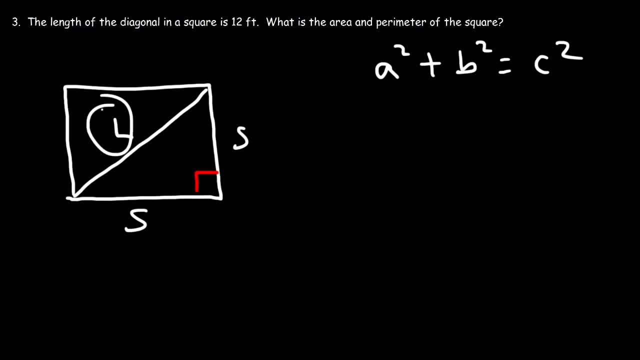 A squared plus B squared equals C squared, where C is the hypotenuse A and B. they're both equal to S. So we have: S squared plus S squared is equal to L squared, And so 1S squared plus 1S squared is 2S squared. 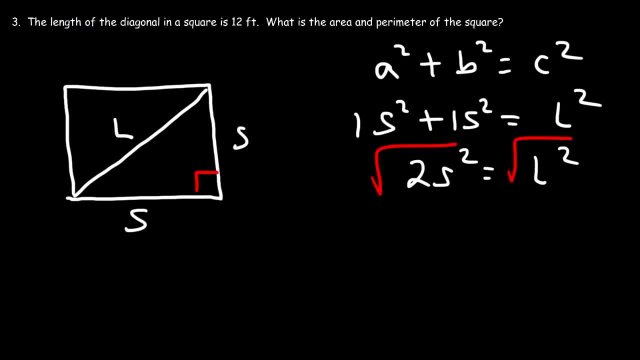 Now, if we take the square root of both sides, on the left we have the square root of 2 times the square root of S squared, And on the right, the square root of L squared is just L And the square root of S squared. we could just make that S. 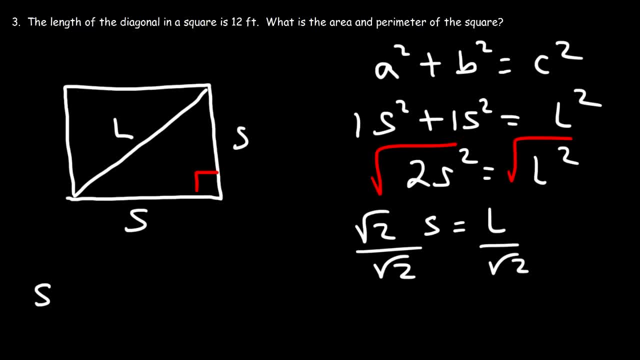 Then we could divide by the square root of 2.. So the side length is basically the length of the diagonal divided by the square root of 2. when dealing with a square Now, the area of a square is S squared, And so what we could do is replace S with this expression. 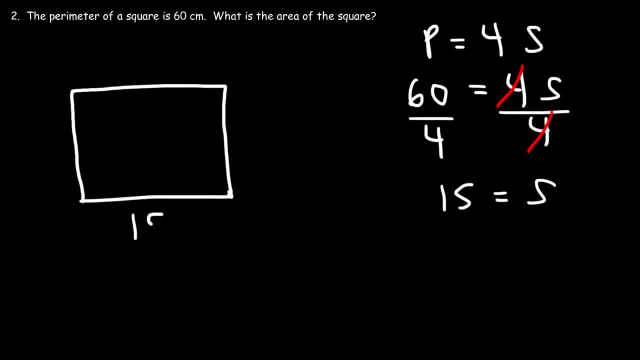 So, therefore, the side length of the square is 15 centimeters all around. So now that we have the side length, we can calculate the area. So the area of this square is going to be S squared, Or basically 15 times 15, which is 15 squared. 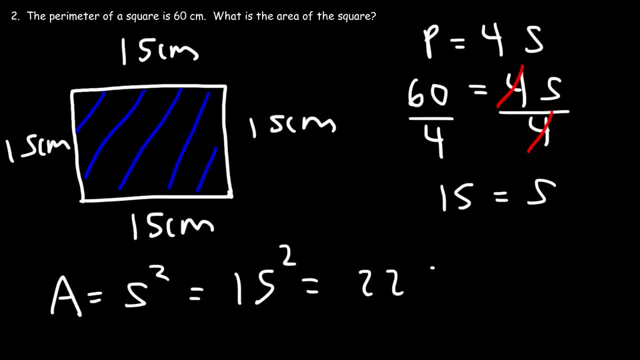 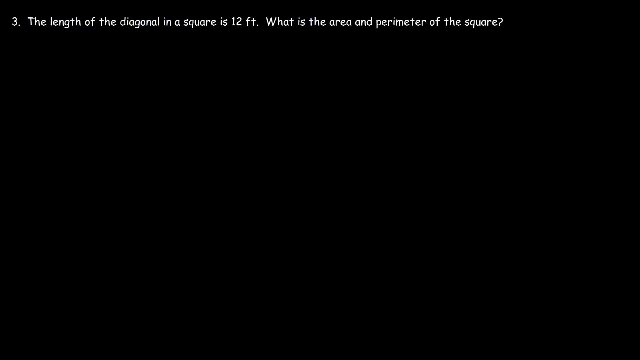 And so that comes out to be 225 square centimeters. And so that's it for this problem. That's the area. That's the area of this particular square. Now let's try this problem. The length of the diagonal in a square is 12 feet. 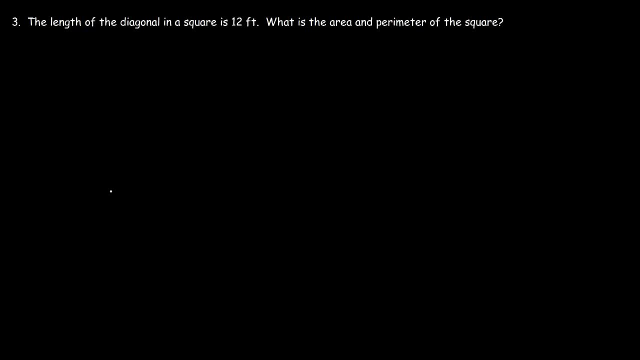 What is the area and perimeter of the square? So, if we're given the length of the diagonal- let's call it L- How can we find the side length S? Let's call it S. Let's call it S. Notice that this forms a right triangle. 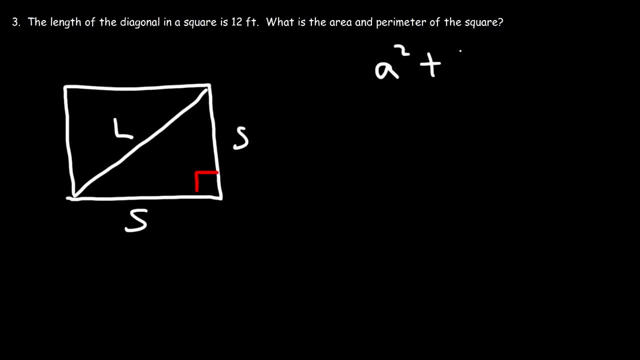 And so we could use the Pythagorean theorem: A squared plus B squared equals C squared, where C is the hypotenuse A and B. they're both equal to S. So we have S squared plus S squared is equal to L squared. 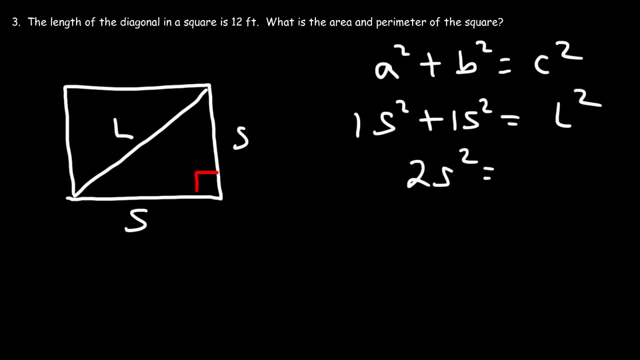 And so 1S squared plus 1S squared is 2S squared. Now, if we take the square root of both sides, on the left we have the square root of 2 times the square root of S squared, And on the right, the square root of L squared is just L. 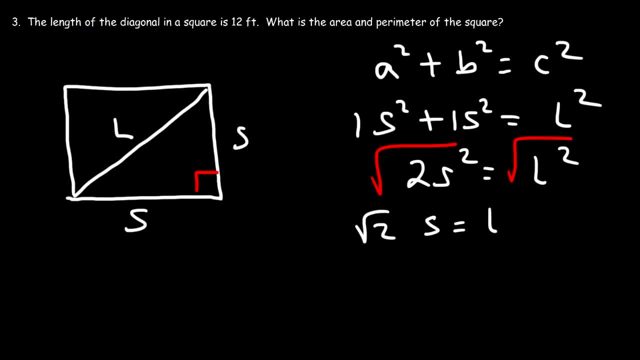 And the square root of S squared, we could just make that S. Then we could divide by the square root of 2.. So the side length is basically the length of the diagonal divided by the square root of 2. when dealing with a square, 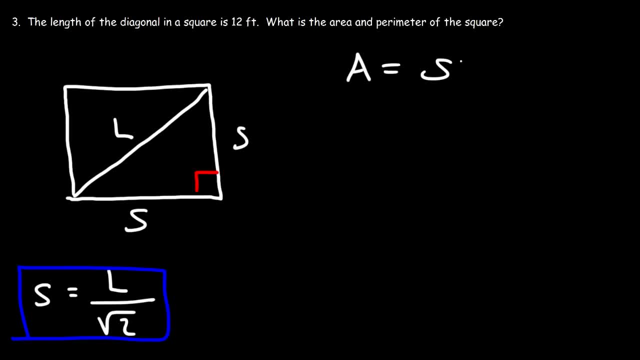 Now the area of a square is S squared, And so what we could do is replace S with this expression. So the area is going to be L over the square root of 2 times- I mean to the second power, And so here we have L squared. 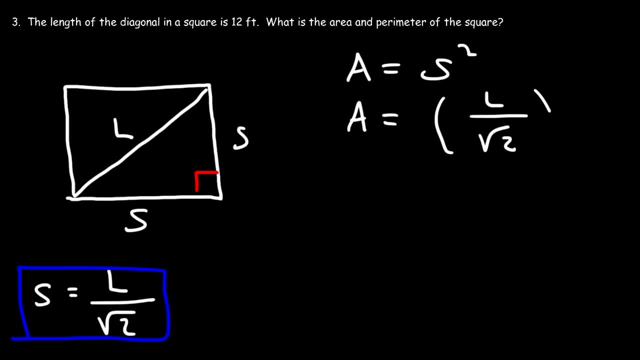 So the area is going to be L over the square root of 2 times, I mean to the second power. And so here we have L squared And then the square root of 2 squared. the square and the square root will cancel. 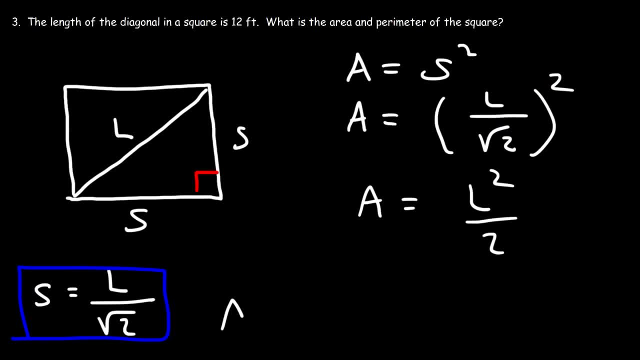 And so you're just going to get a 2 on the bottom. Therefore, the area of a square, given the left of the diagonal, is 1 half L squared, And so let's use that formula to get the area of this square. So the left of the diagonal is 12, and 12 squared is 144.. 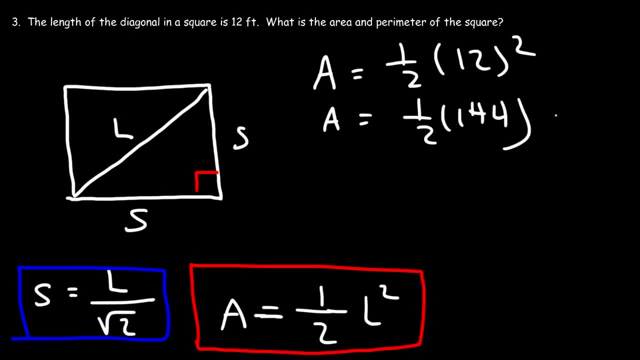 Half of 144,. well, half of 14 is 7, and then half of the other 4 is 2, so half of 144 is 72.. So it's going to be 72 square feet And that's going to be the area of the diagonal. 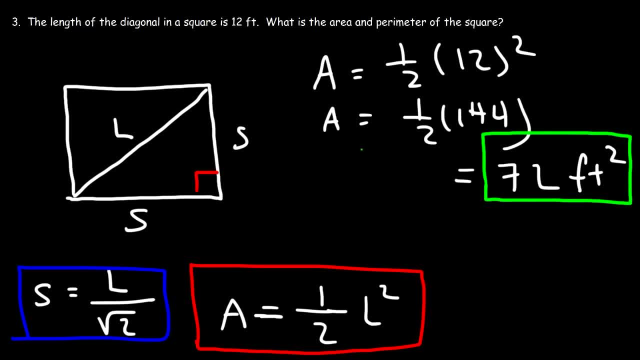 And that's the area of this particular square. Now let's calculate the perimeter of the square. So the perimeter of the square, we know it's 4S And in this problem, S is L over the square root of 2.. 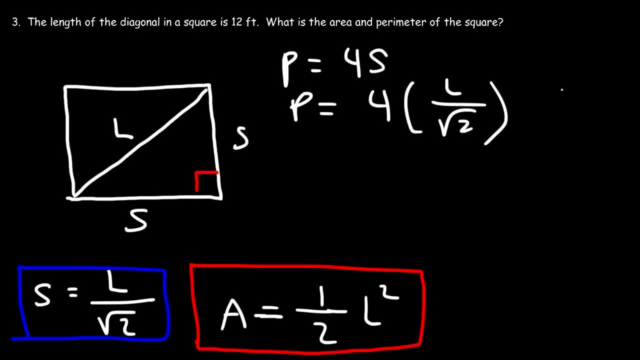 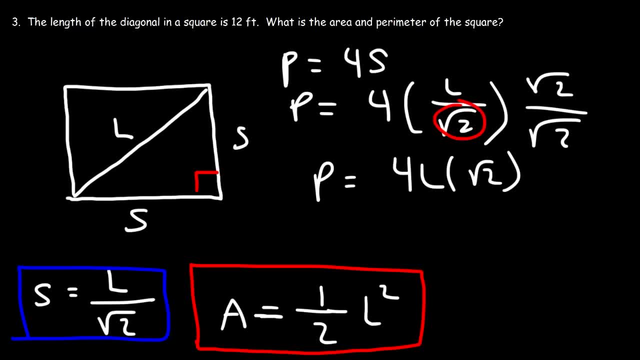 On top I have 4L And on the bottom the square root of 2 times the square root of 2, that's the square root of 4, which is 2.. And now 4 divided by 2 is 2.. 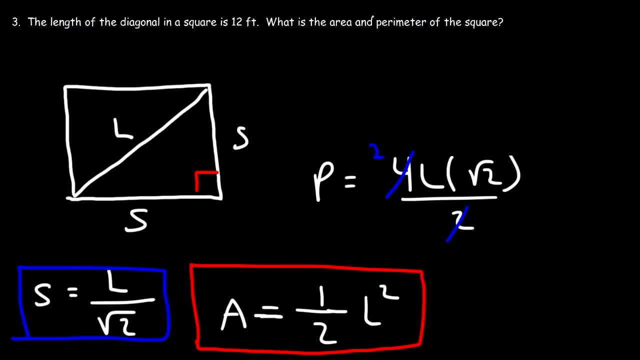 So you could simplify these. replace that with a 2.. So, in terms of the length of the diagonal, the perimeter of the square is going to be 2L, or rather 2L. So, in terms of the length of the diagonal, the perimeter of the square root of 2 is 2L. 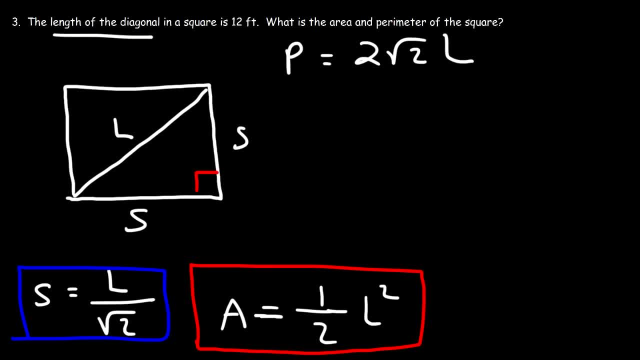 So, in terms of the length of the diagonal, the perimeter of the square root of 2 is 2L, So in this case it's going to be 2 square root 2 times 12. Or basically, 24 square root 2.. 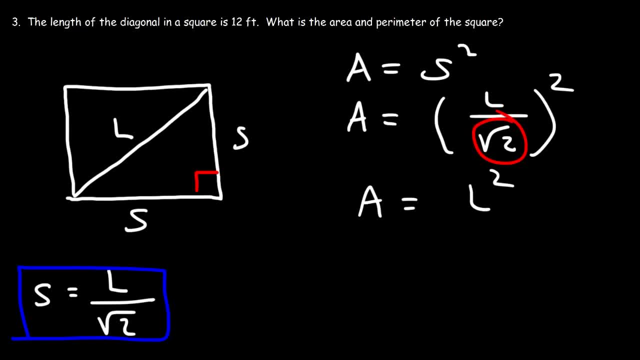 And then the square root of 2 squared, The square and the square root will cancel, And so you're just going to get a 2 on the bottom. Therefore, the area of a square, Given the length of the diagonal, is 1 half L squared. 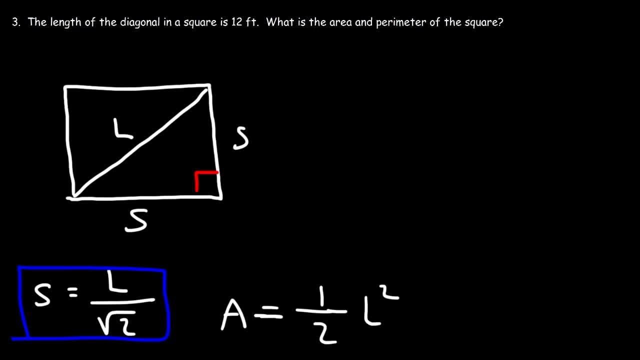 And so let's use that formula to get the area of this square. So the length of the diagonal is 12. And 12 squared is 144.. Half of 144.. Well, half of 14 is 7., And then half of the other 4 is 2.. 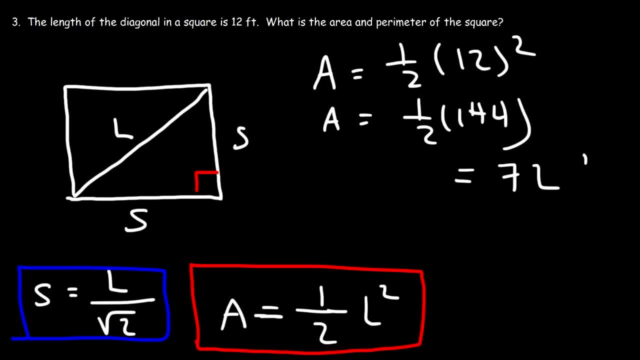 So half of 144 is 72.. So it's going to be 72 square feet And that's the area of this particular square. Now let's calculate the perimeter of the square. So the perimeter of the square, we know it's 4S. 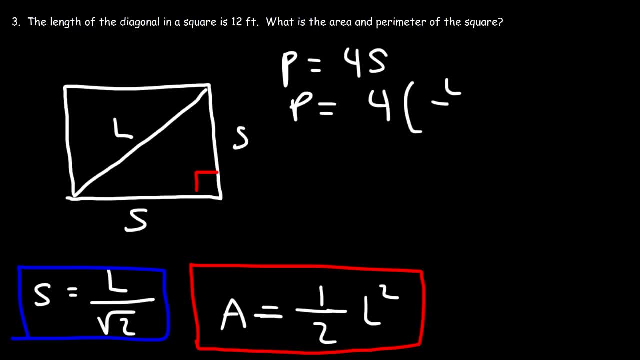 And in this problem, S is the area of the square, S is L over the square root of 2.. So now I'm going to rationalize this expression. I'm going to multiply the top and the bottom by the square root of 2.. 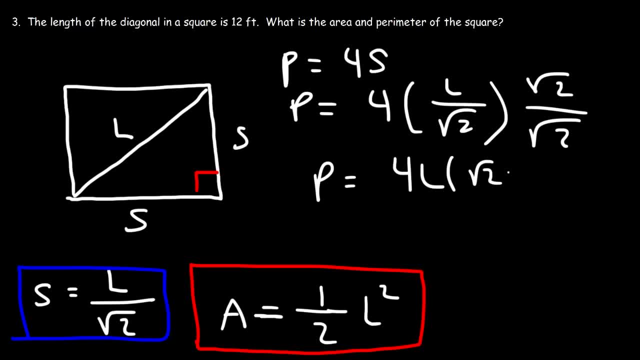 So on top I have 4L times the square root of 2. And on the bottom the square root of 2 times the square root of 2.. That's the square root of 4, which is 2.. And now 4 divided by 2 is 2.. 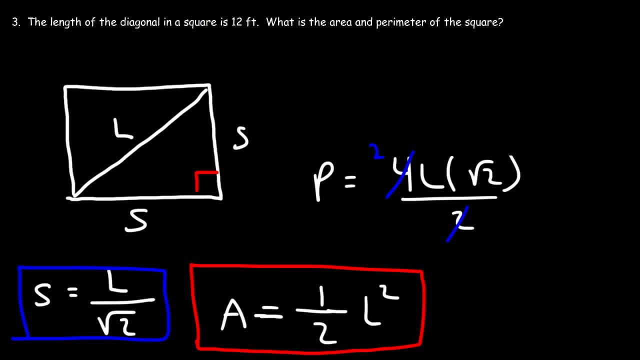 So you can simplify these. replace that with a 2.. So, in terms of the length of the diagonal, the perimeter of the square is going to be 2L, or rather 2 square root 2 times L. So in this case it's going to be 2 square root 2 times 12.. 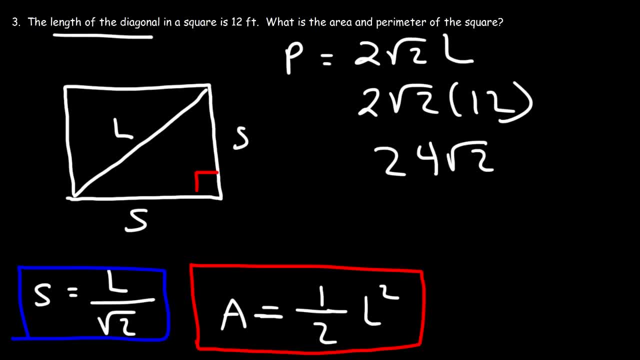 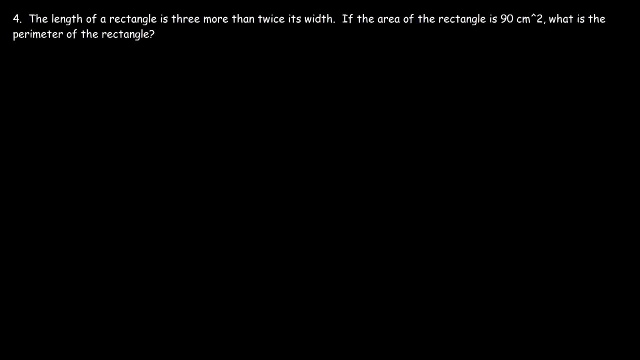 Well, basically, 24 square root 2. And the unit for this is 4L feet, so that's the perimeter of this particular square. so this problem is going to be the last problem for this video. so it goes like this: the left of a 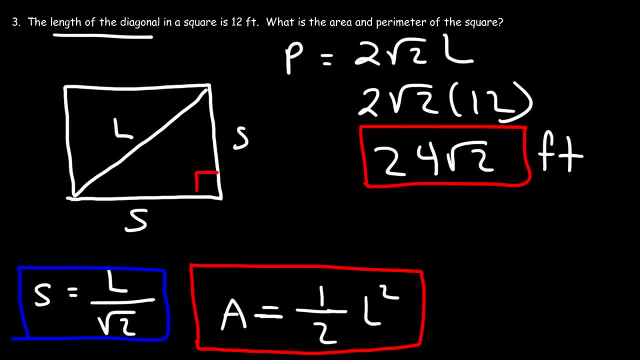 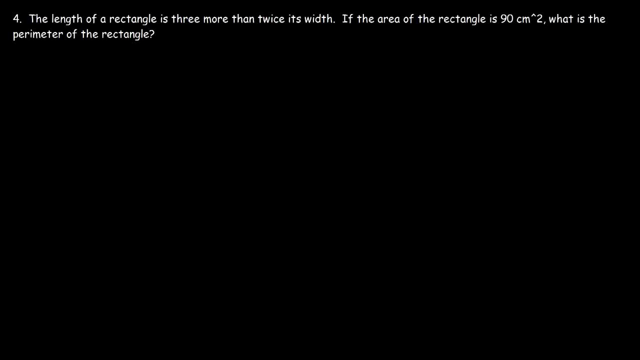 And the unit for this is feet, So that's the perimeter of this particular square. So this problem is going to be the last problem for this video. So it goes like this: The left of a rectangle is 2.. So it goes like this: 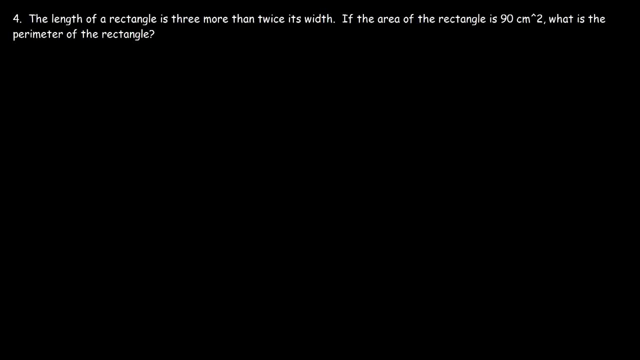 The left of a rectangle is 4.. three more than twice its width. If the area of the rectangle is 90 square centimeters, what is the perimeter of the rectangle? So let's draw a picture, And so this is the length and this is the width. Now what we need to do is we need to. 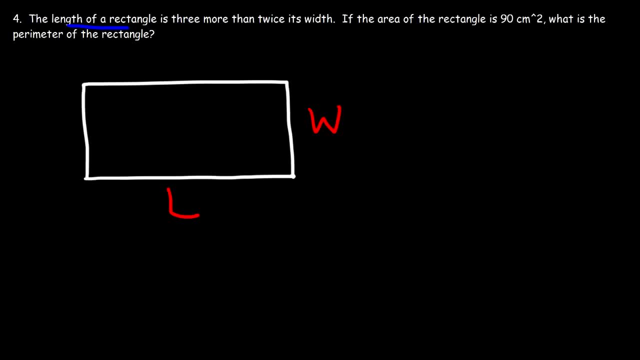 write some equations. We're told that the length of the rectangle is three more than twice its width. How can we convert that sentence into an equation? So the left is: is means equal three more. so three plus twice the width, 2w. Now we're. 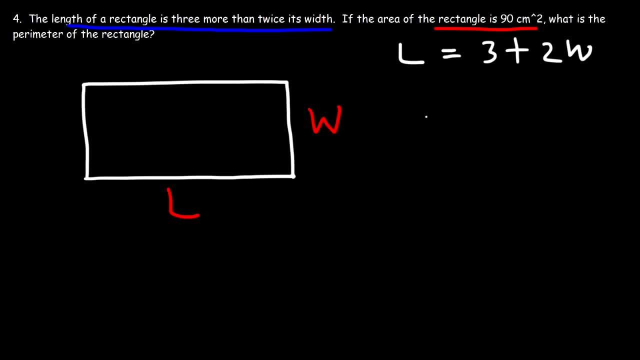 also told that the area is 90 square centimeters and we know that the area is left times width, so 90 is L times W. So we have two equations and two variables. So let's solve by substitution. So let's replace L with 3. 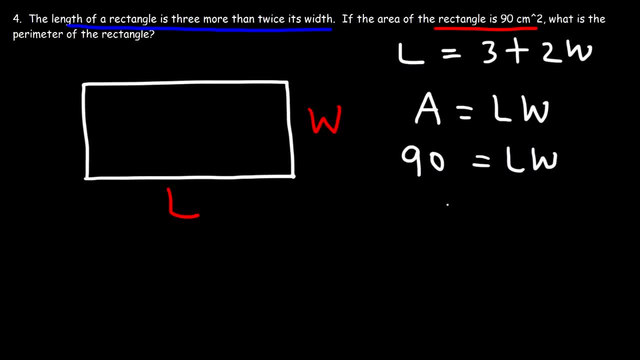 plus 2w. So this is going to be: 90 is equal to 3 plus 2w times W. So now we have an equation with only one variable, so we can solve it. But how should we go about solving it? Well, the first thing we should do is distribute W to three. 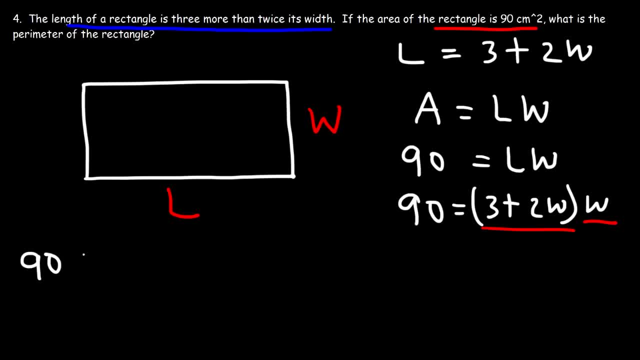 plus 2w, And so it's going to be: 90 is equal to 3 times W, which is 3w, and then 2w times W, that's 2w squared, And so I'm going to take this 90 and move it to. 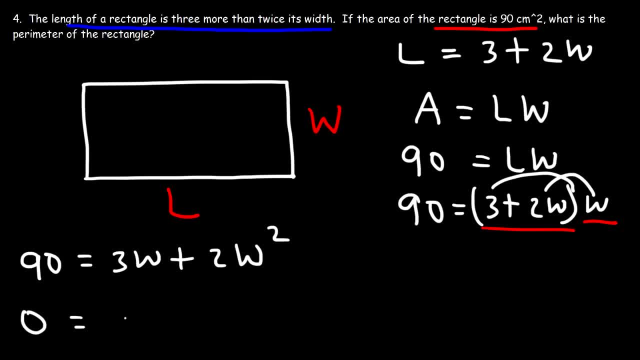 that side And I'm going to rewrite it, putting it in standard order. So it's 2w squared plus 3w, and then when you take the 90, which is positive on the left side- and move it to the right side, it's going to switch from positive to negative. 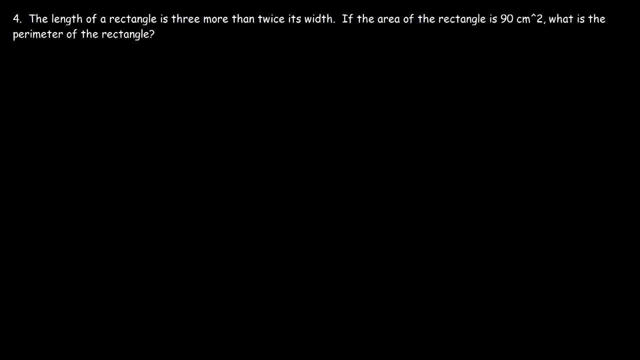 rectangle is three more than twice its width. if the area of the rectangle is 90 square centimeters, what is the perimeter of the rectangle? so let's draw a picture, and so this is the left and this is the width. now what we need to do is we need to write some 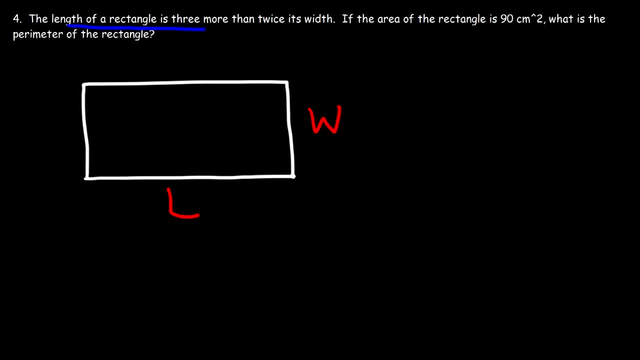 equations were told that the left of the rectangle is three more than twice its width. how can we convert that sentence into an equation? so the left is is means equal three more, so three plus twice the width: 2w. now we're also told that the area is 90 square centimeters, and we know that the 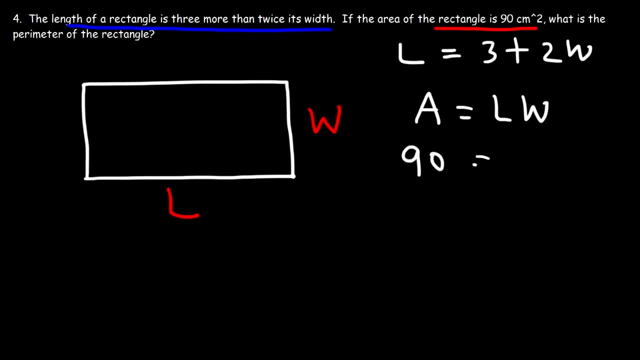 area is left times with. so 90 is L times W. so we have two equations and two variables. so let's solve by substitution. so let's replace out with 3 plus 2w. so this is going to be: 90 is equal to 3 plus 2w times W. 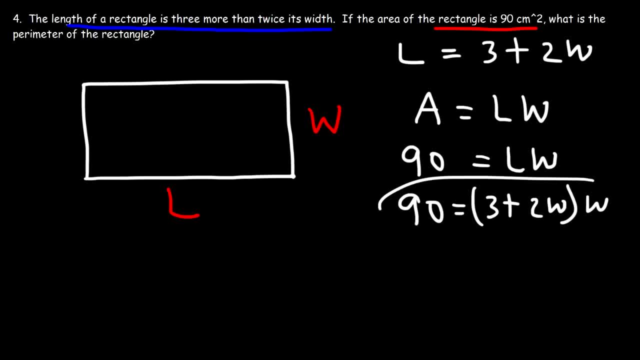 so now we have an equation with only one variable, so we can solve it. but how should we go about solving it? well, the first thing we should do is distribute w-2, 3 plus 2 w, and so it's going to be: ninety is equal to three times w, which is 3 w, and then 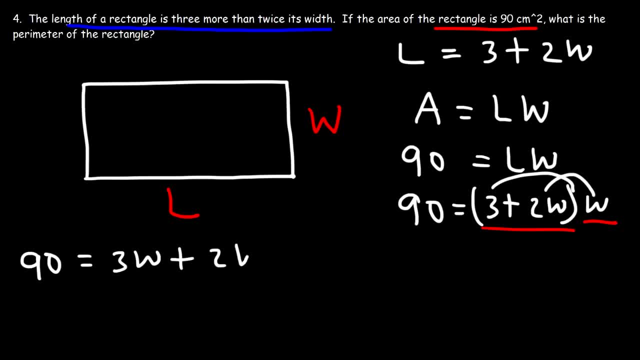 2w times W, that 2w square, and so I'm going to take this 90 and move to that side and I'm going to rewrite it, putting it in standard order. So it's 2w squared plus 3w. and then when you take the 90, which is 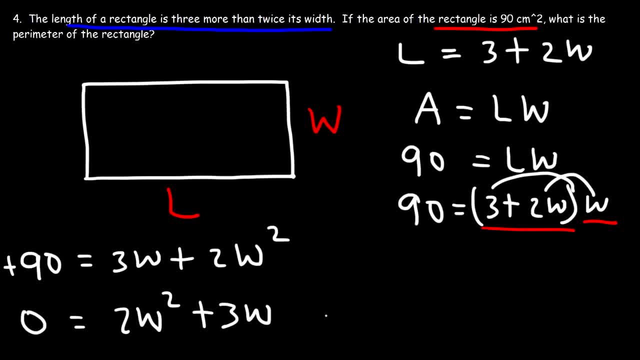 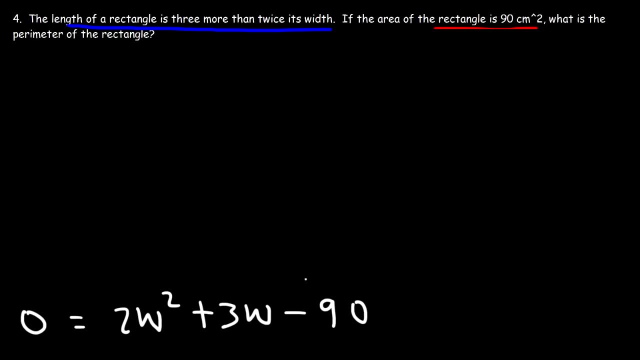 positive on the left side and move it to the right side. it's going to switch from positive to negative. Now, in order to solve for w, we either need to factor or use the quadratic formula, Because right now this is a quadratic equation. Let's see if we can. 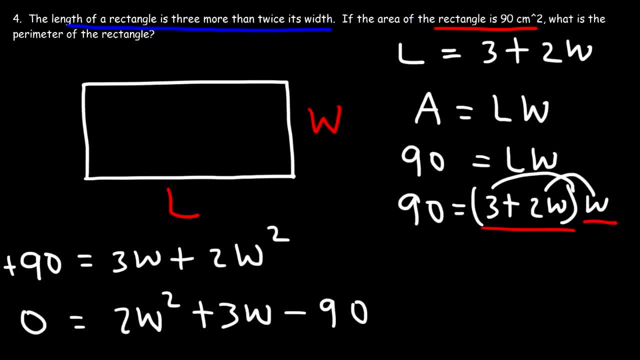 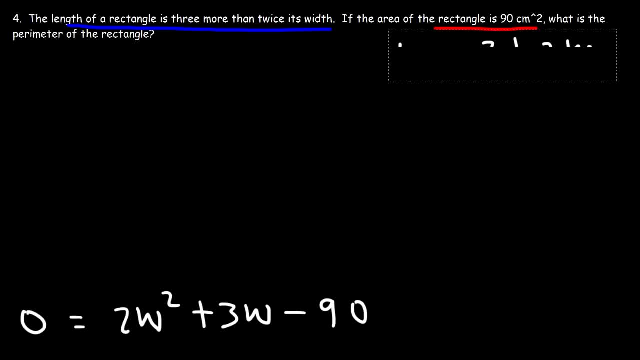 Now, in order to solve for W, we either need to factor or use the quadratic formula, Because right now this is a quadratic equation. Let's see if we can factor. So first we need to multiply the leading coefficient by the constant term, 2 times negative. 90 is negative 180. And now we need to find two numbers that 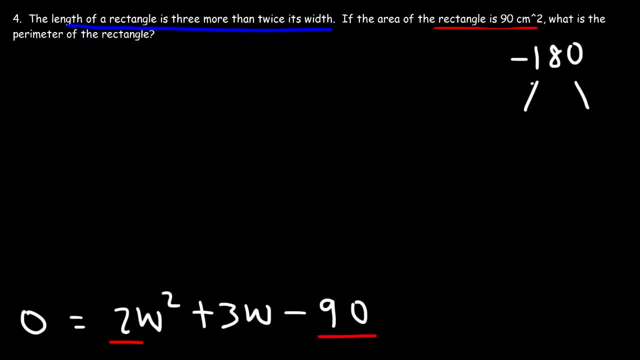 multiply to negative 180.. 80, but add to 3, so we could try negative 18. negative 180 divided by negative 18 is 10, but these two numbers, they don't differ by 3, so we could try, let's say, 6. 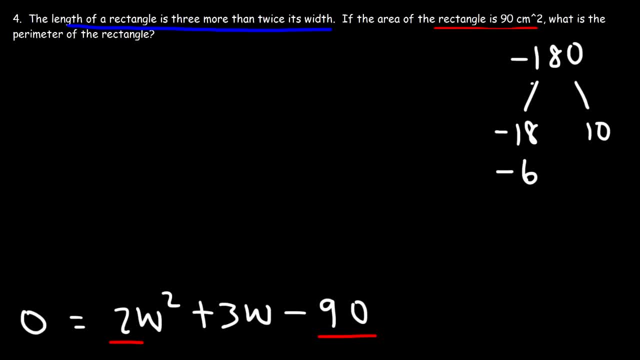 goes into 18. negative 180 divided by 6, or negative 6, that's 30, but they don't differ by 3. we could try: negative 12, negative 180 divided by negative 12, that's 15. so these two, they differ by 3. so what we're going to do is we're going. 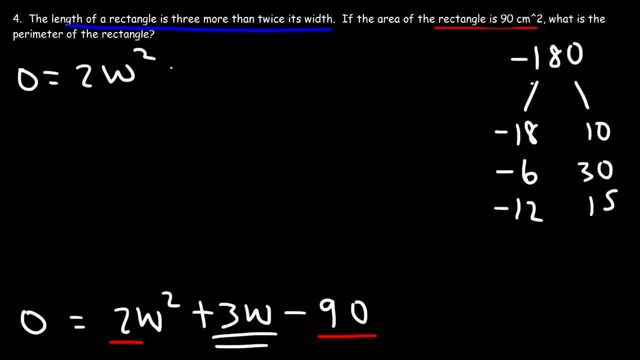 to replace the middle term 3 W with negative 12 W plus 15 W, because, as you can see, these two numbers, they add up to 3 W, you. and now let's factor by grouping. so in the first two terms let's take out the: 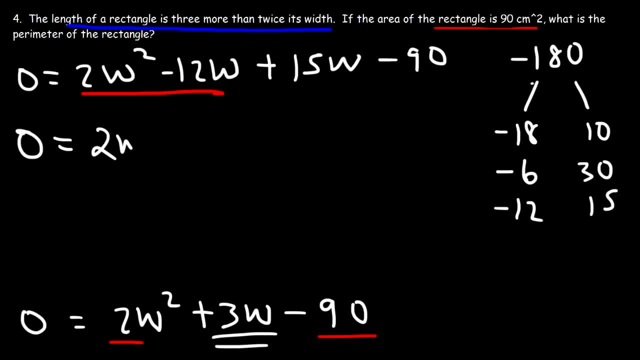 GCF, the greatest common factor, which is 2 W. and so now we have 2 W squared divided by 2 W, which is W, and then negative 12 W divided by 2 W, that's going to be negative 6, and the last two terms, let's factor out the greatest. 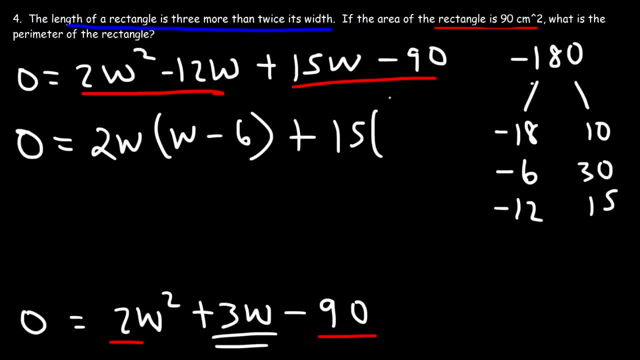 common factor, which is going to be 15. and so 15 W divided by 15, that's going to be just W negative 90 divided by 15, that's negative 6, and so at this point you can see we have a common factor, and so if we take out W, 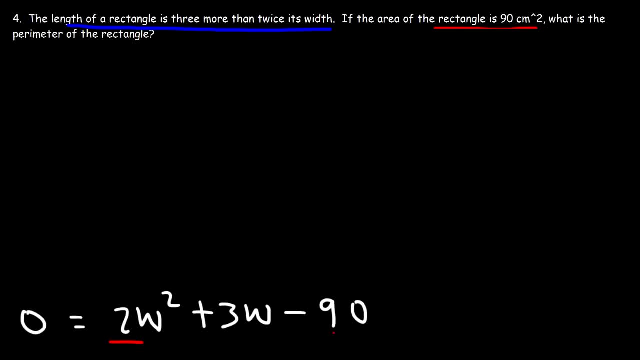 factor. So first we need to multiply the leading coefficient by the constant term. 2 times negative 90 is negative 180. And now we need to find two numbers that multiply to negative 180, but add to 3. So we could try negative 18.. Negative 180 divided by negative. 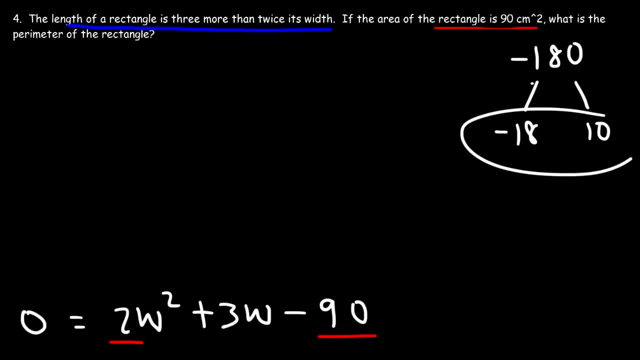 18 is 10.. But these two numbers, they don't differ by 3.. So we could try, let's say 6 goes into 18.. Negative 180 divided by 6, or negative 6,, that's 30. But they don't differ. 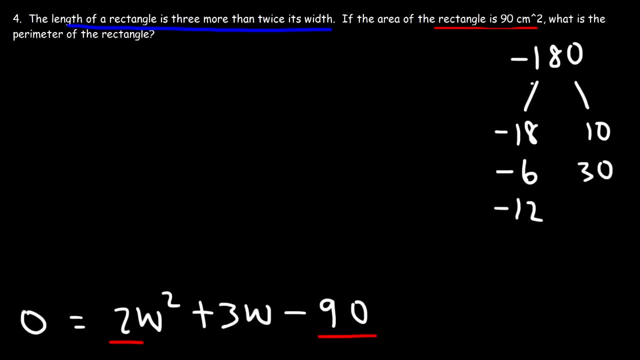 by 3.. We could try negative 12.. Negative 180 divided by negative 12, that's 15.. So these two, they differ by 3.. So what we're going to do is we're going to replace the middle. 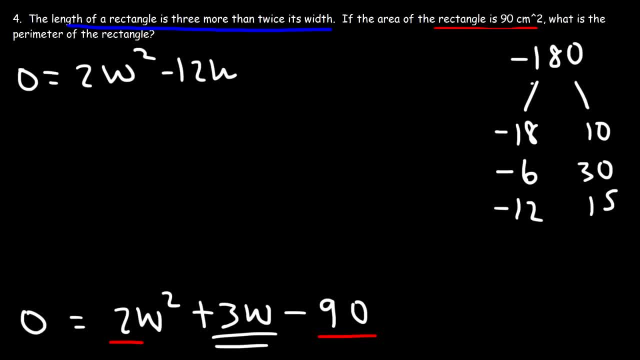 term 3w, with negative 12w plus 15w, Because, as you can see, these two numbers, they add up to 3w. And now let's factor by grouping. So in the first two terms let's take out the GCF, the greatest common factor, 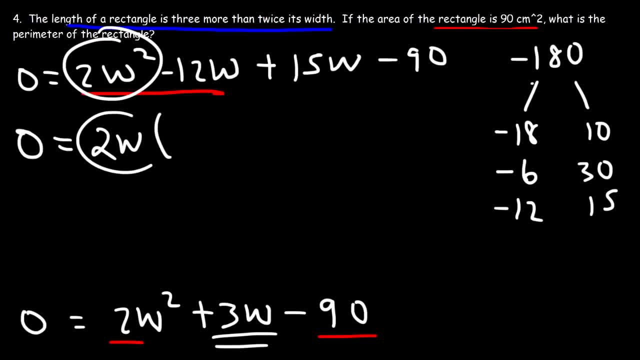 which is 2w. And so now we have 2w squared divided by 2w, which is w, And then negative 12w divided by 2w, that's going to be negative 6.. And the last two terms let's factor out. 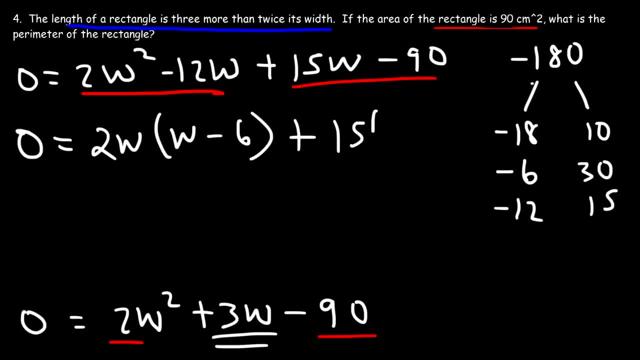 the greatest common factor, which is going to be 15.. And so 15w divided by 15,, that's going to be just w Negative. 90 divided by 15,, that's negative 6.. And so, at this point, 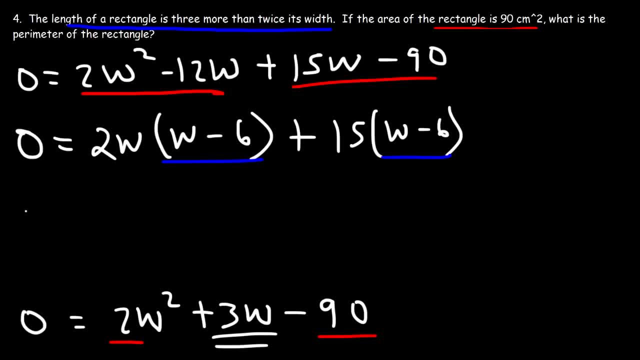 you can see, we have a common factor, And so if we take out w minus 6,, we will be left over with 2w plus 15.. And so at this point we can now calculate the value of w, And so we need to set each.